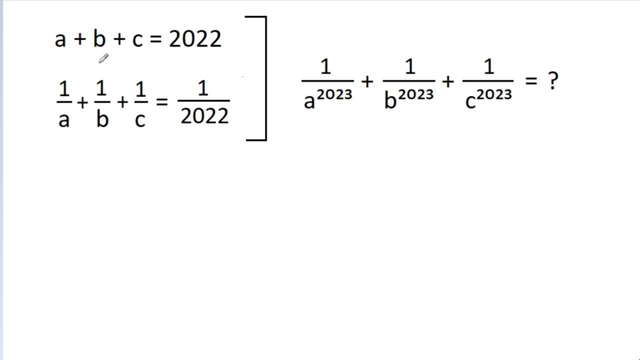 In this video we have given that a plus b plus c is equal to 2022, and 1 by a plus 1 by b plus 1 by c is equal to 1 by 2022.. Then we have to find the value of 1 by a- power 2023- plus 1 by b- power 2023- plus 1 by c- power 2023. 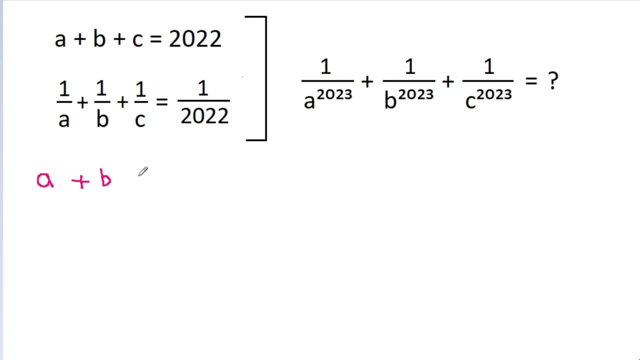 So we have a plus b plus c is equal to 2022. And 1 by a plus b plus c will be equal to 1 by, and a plus b plus c is 2022. And also we have given that 1 by a plus 1 by b plus 1 by c is equal to 1 by 2022. 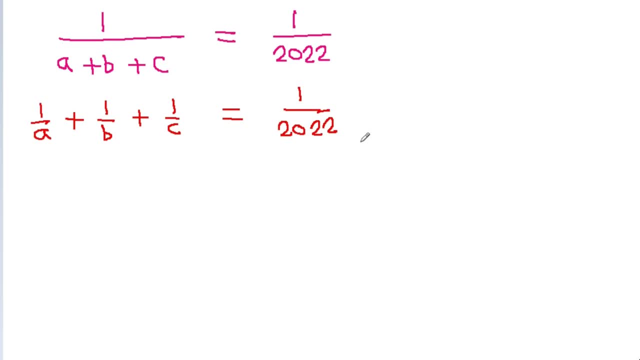 So So From these two equations We can get: 1 by a plus b plus c is equal to 1 by a plus 1 by b plus 1 by c, And 1 by a plus b plus c minus 1 by a plus 1 by c is equal to 22.. 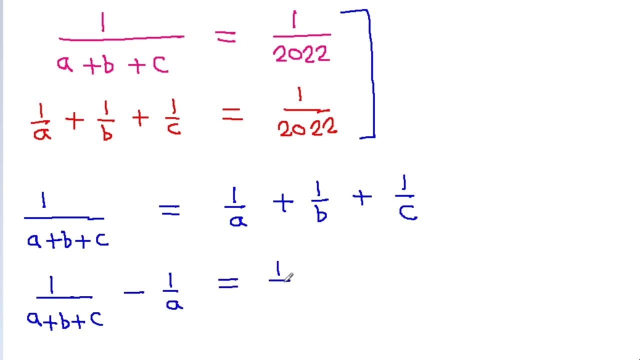 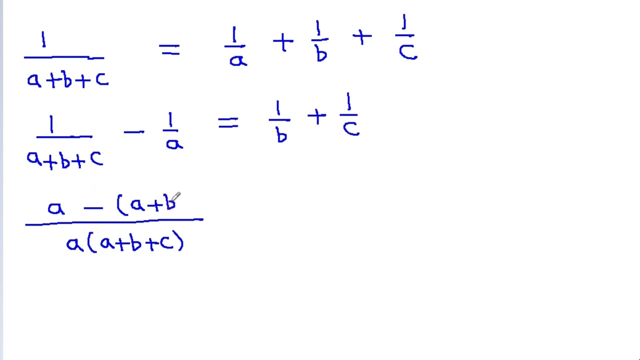 1 by A will be equal to 1 by B plus 1 by C, and here A times A plus B plus C will be NCM and we will get A minus A plus B plus C is equal to, and here BC will be NCM and we will get C plus B and A will get constant. So minus of B plus C by A. 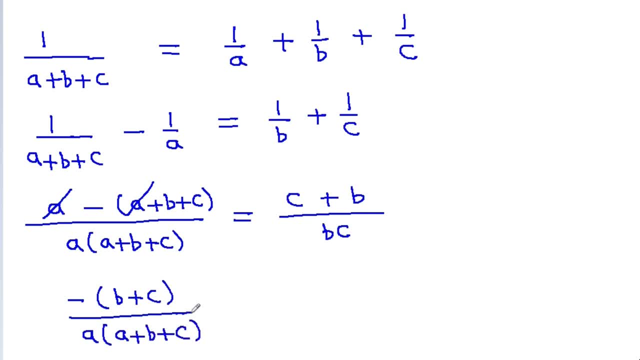 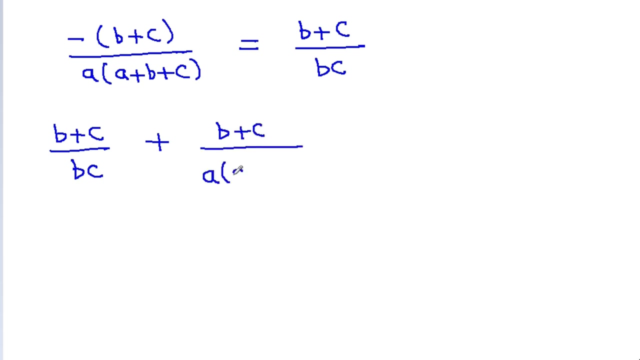 times A plus B plus C is equal to b plus c by bc, and it is b plus c by bc plus b plus c by a. times a. a plus b plus c is equal to zero. and we can take b plus c common and we will get 1 by bc. 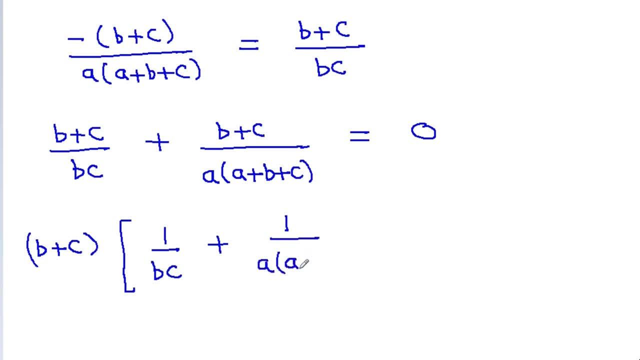 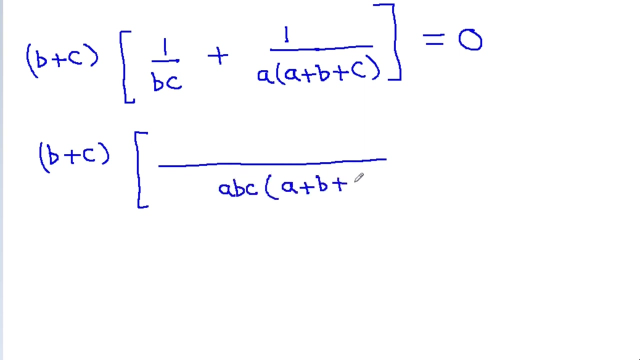 plus 1 by a times a plus b plus c is equal to zero and a times b plus c is equal to zero. it is b plus c times and bc times. a times a plus b plus c will be abc times a plus b plus c, and here we will get a times a plus b plus c plus bc. 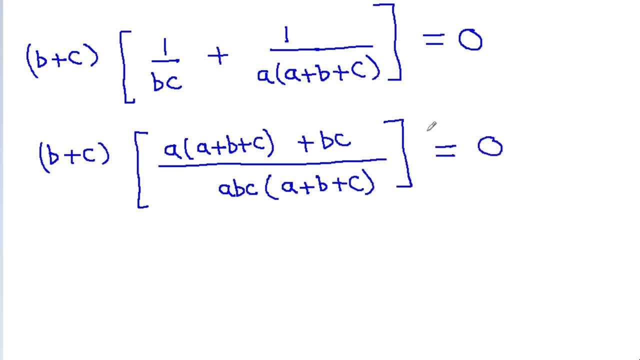 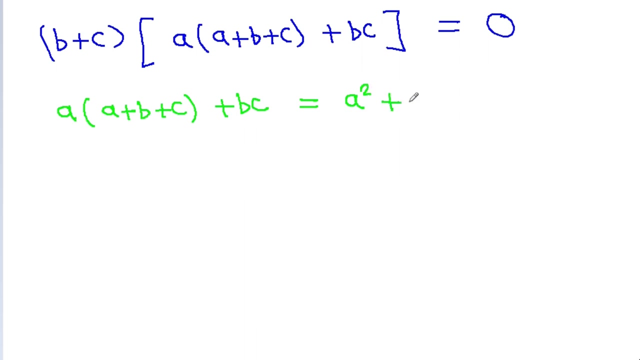 is equal to zero and it is b plus c. times a. times a plus b plus c plus bc is equal to and zero times abc. times a plus b plus c will be zero and a times a times a plus b plus c plus bc, it is a. times a is a square plus a. times b is ab plus a. times c is ac plus bc. 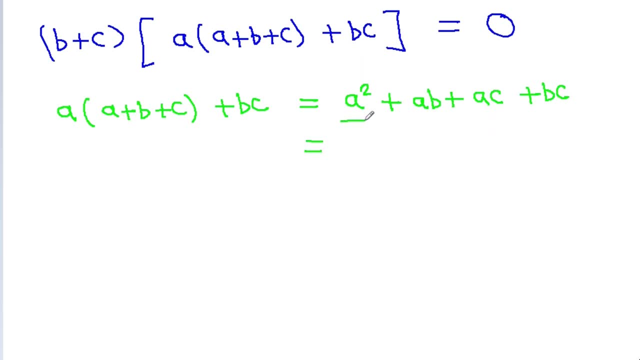 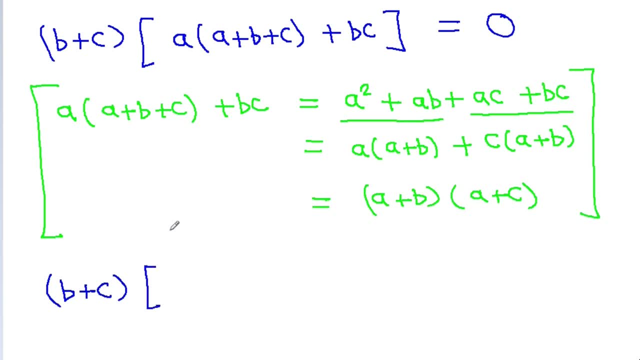 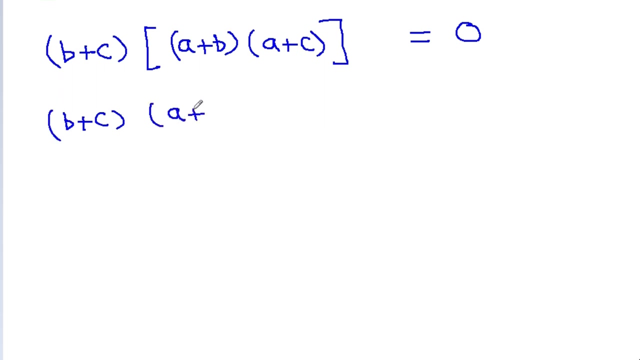 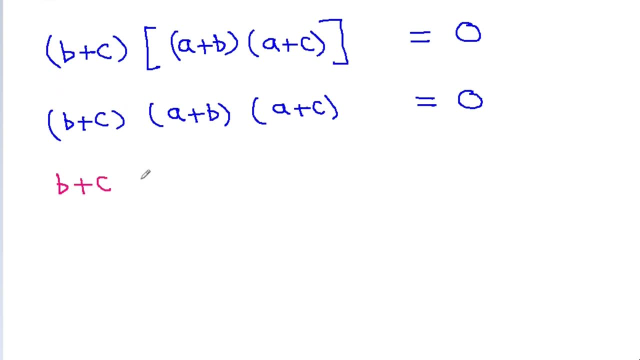 and it is b plus c. times a plus b. times a plus b. times a plus c is equal to zero. and it is b plus c. times a plus b. times a plus b. times a plus b is equal to zero. and it is b plus c. times a plus b. times a plus b. times a plus b is equal to zero. so either b plus c. 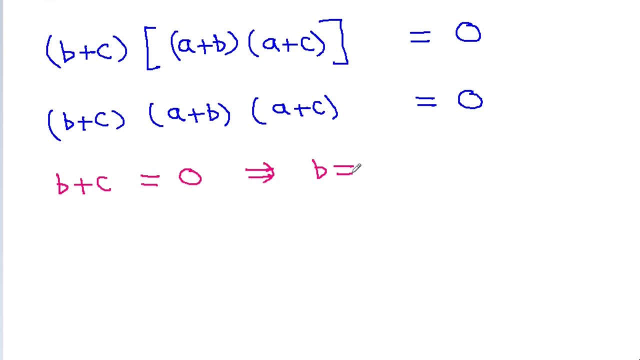 so either b plus c is equal to zero and b is equal to minus c and b is equal to minus c and b is equal to minus c, or a plus b is equal to zero, or a plus b is equal to zero, or a plus b is equal to zero and a is equal to minus b. 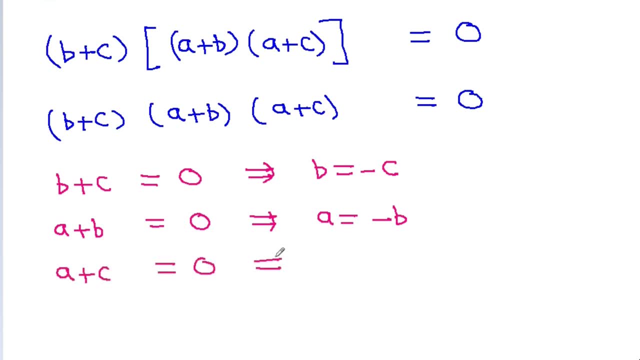 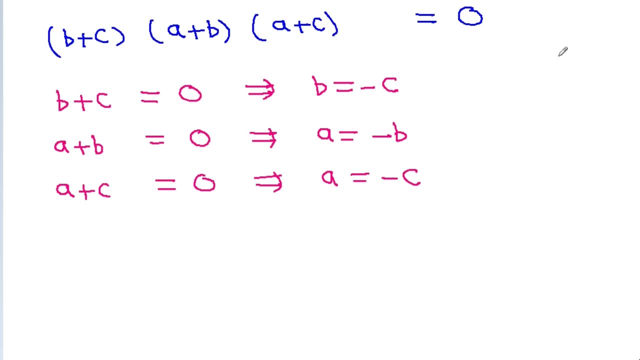 and a is equal to minus b and a is equal to minus b, or a plus c is equal to zero, or a plus b is equal to minus c is equal to zero. we have given that a plus b, we have given that a plus b. we have given that a plus b plus c is equal to 2022. 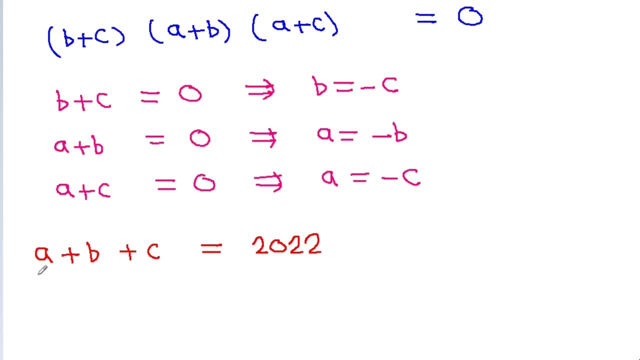 and on the equations asymmetric with, and on the equations asymmetric with, and on the equations asymmetric with respect to a respect to a respect to a, b and c, so b and c, so b and c. so, from a plus b is equal to zero, from a plus b is equal to zero. 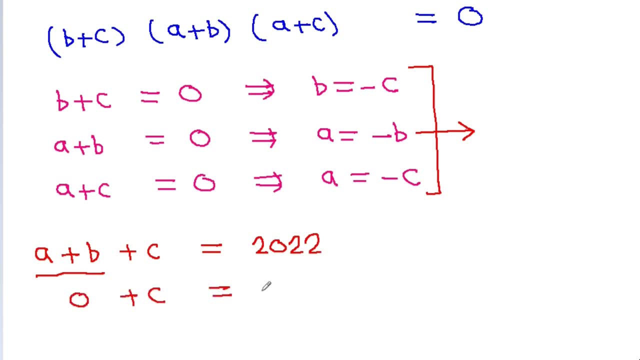 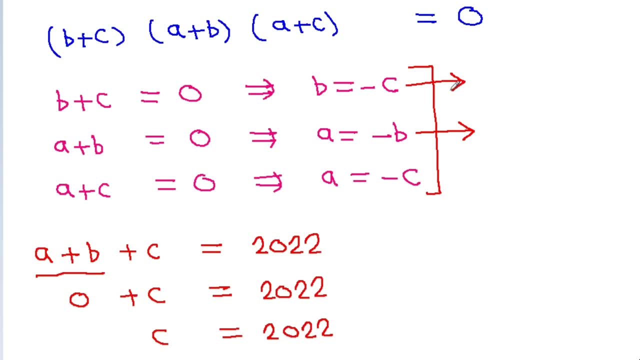 so we can get: c is equal to 2022. so we can get: c is equal to 2022, and from here we can also get a is, and from here we can also get a is, and from here we can also get: a is equal to 2022. 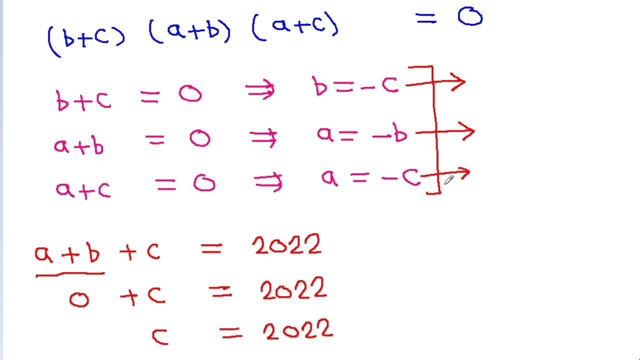 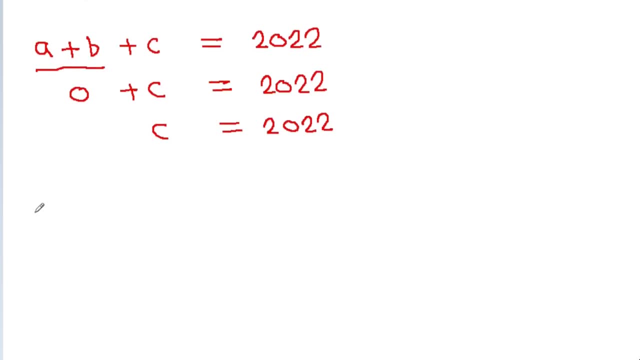 equal to 2022, equal to 2022, and from here we can get: b is equal to, and from here we can get: b is equal to, and from here we can get: b is equal to 2022, and we have to find the value of 1 by. 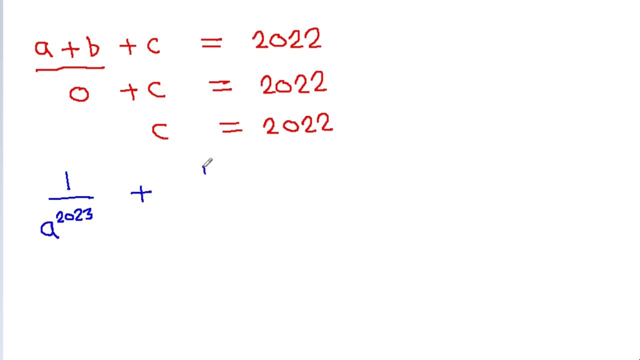 we have to find the value of 1 by. we have to find the value of 1 by a power 2023, a power 2023, a power 2023 plus 1 by plus 1 by, plus 1 by a power 2023 plus 1 by. 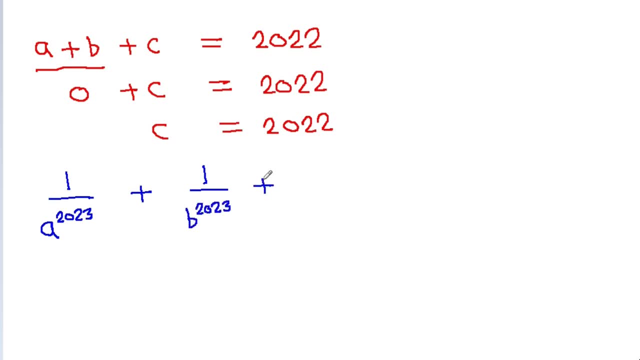 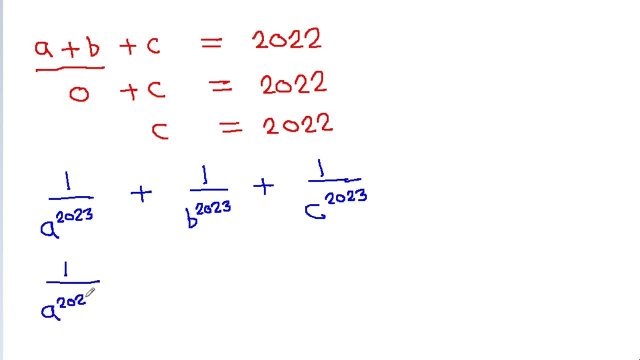 and it is 1 by and it is 1 by. and it is 1 by: a power 2023: a power 2023- a power 2023 plus 1 by plus 1 by plus 1 by. and b is minus a and b is minus a. 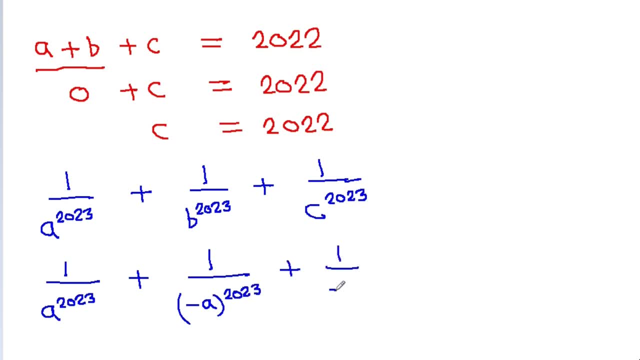 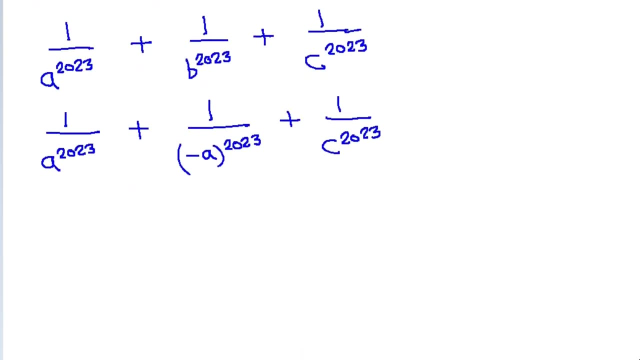 and b is minus a power 2023: power 2023: power 2023 plus 1 by c- power 2023. plus 1 by c- power 2023 plus 1 by c- power 2023, and and and and minus a power 2023. 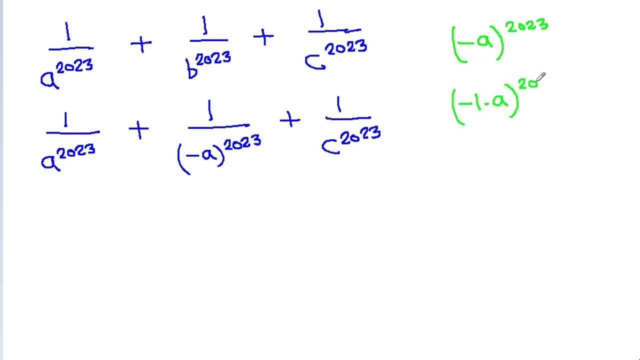 minus a power 2023. it is minus 1 times a minus a power 2023. it is minus 1 times a minus a power 2023. it is minus 1 times a power 2023. power 2023, power 2023. and it is minus 1 power 2023. 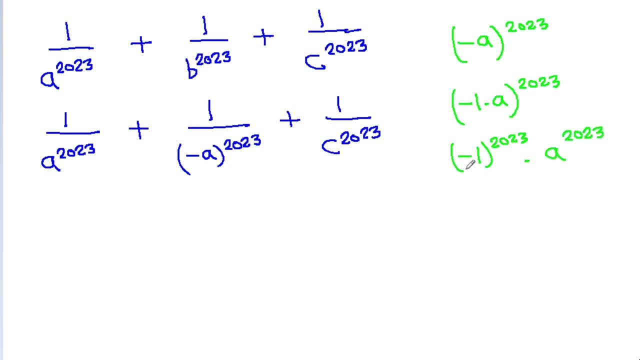 and it is minus 1. power 2023, and it is minus 1 power 2023 times a power 2023. times a power 2023- times a power 2023. and minus 1 power 2023 will be minus 1. 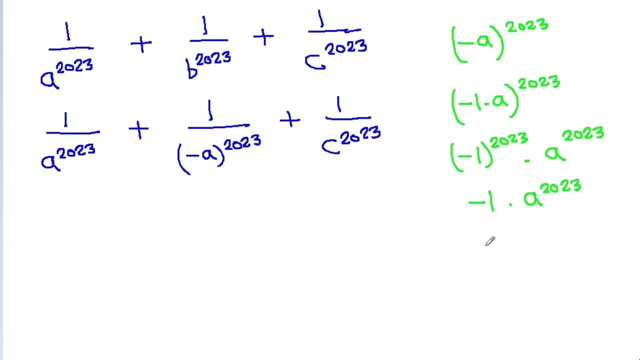 and minus 1 power 2023 will be minus 1 and minus 1 power 2023 will be minus 1 times a power 2023. times a power 2023, and it is minus a and it is minus a power 2023 and it is minus a. 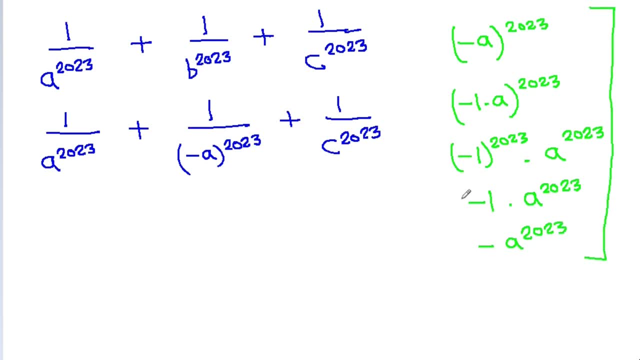 and it is minus a power 2023, and it is minus a power 2023, power 2023. so it is 1 by, so it is 1 by, so it is 1 by a power 2023, a power 2023, a power 2023, and this is minus. 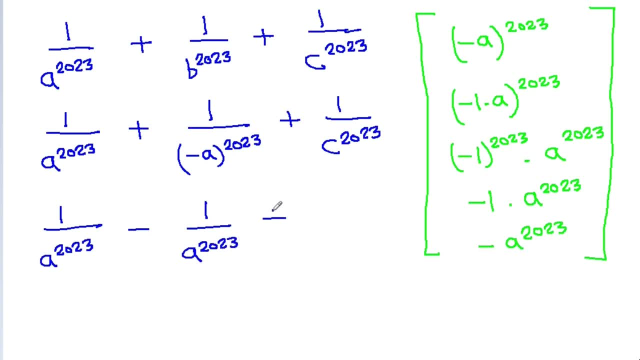 and this is minus and this is minus: 1 by a power 2023. 1 by a power 2023. 1 by a power 2023 plus 1 by plus. 1 by plus 1 by c power 2023. c power 2023.